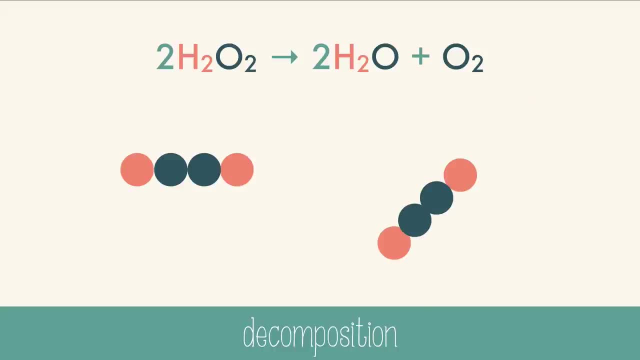 an example of hydrogen peroxide breaking down into water and oxygen. Usually, decomposition reactions need heat or fire or electricity to get started. This reaction can happen quickly, just like yeast or manganese dioxide. So we have the equation, a drawing and now a simple formula for decomposition. AB yields A plus B. The resulting compounds are smaller. 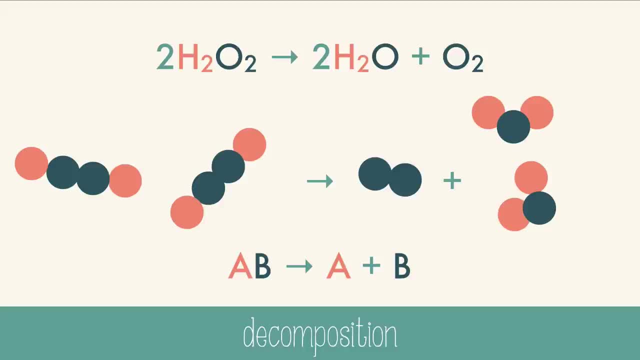 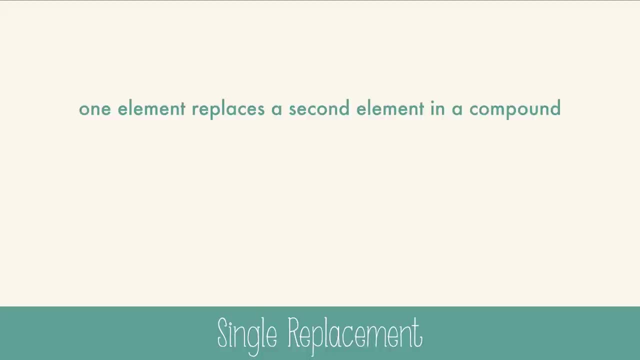 and simpler than the starting compound. Let's look at the next type of reaction: Single replacement. In this reaction, one element replaces a second element in a compound. We'll use the example of zinc reacting with iron chloride to make zinc chloride and elemental. 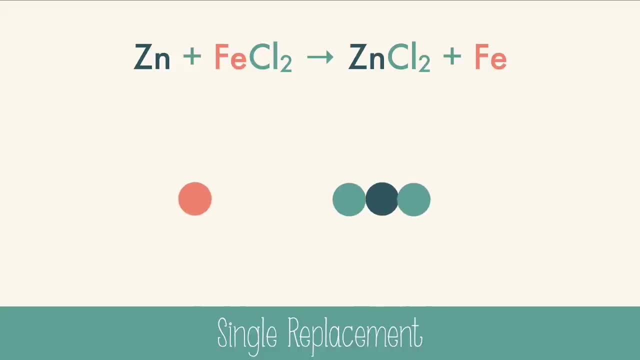 iron. The two metals in this reaction are zinc chloride and elemental iron. The two metals in this case have swapped places. So here we have an equation, a drawing and now a simple formula for single replacement reactions. A plus BC yields AC plus B, But not all single. 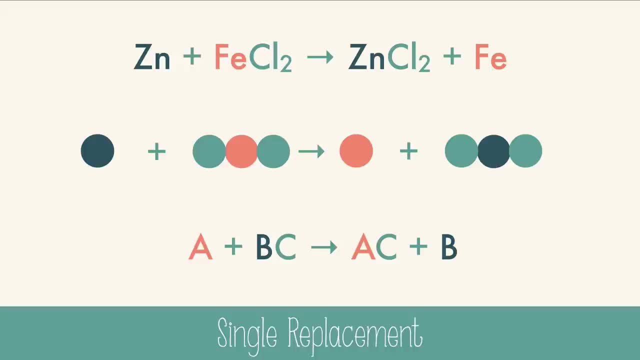 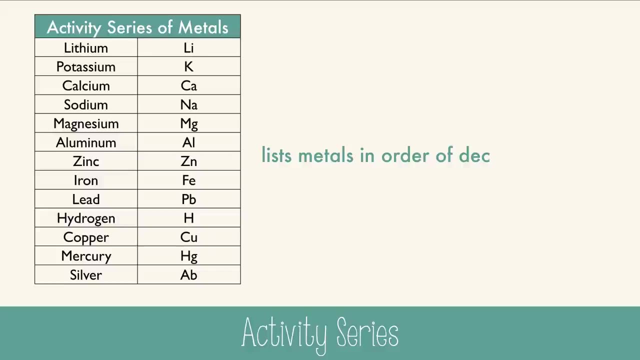 replacement scenarios actually work. In order to see if the swap will occur, we need to reference a chart, the activity series of metals. The more active metals are toward the top and metals decrease in their activity as you move to the bottom. In the previous 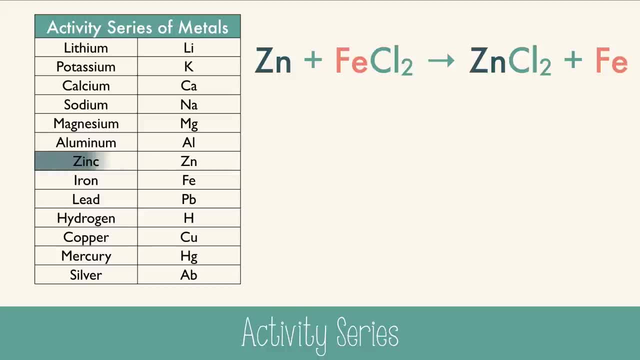 reaction. zinc was the individual element and it was higher than the active element, So this reaction occurred. But if we tried to react elemental iron with zinc chloride, nothing would happen because iron has a lower activity than zinc. Now let's look at the next type of reaction: Double replacement. This reaction is similar. 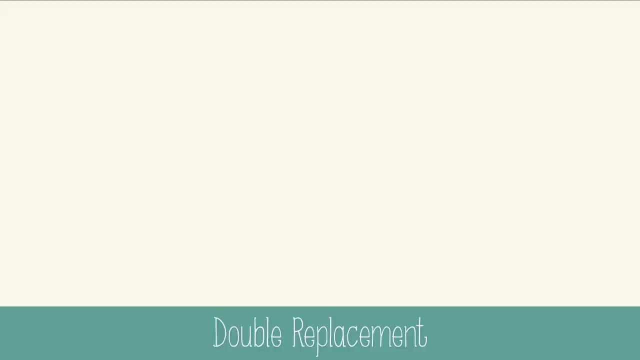 to single replacement, except we're starting with two compounds. The reaction has an exchange of positive ions between two compounds. In this example, copper chloride and hydrosulfuric acid will swap their positive ions to make copper sulfide and hydrochloric acid. 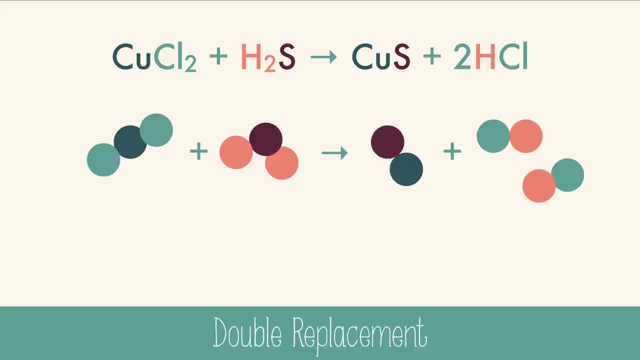 So here we have an equation, a drawing and now a simple formula for single replacement reactions. AB plus CD yields AD plus CB. You can see from this equation that A and C have just switched places and those represent the positive ions, Usually a double replacement.